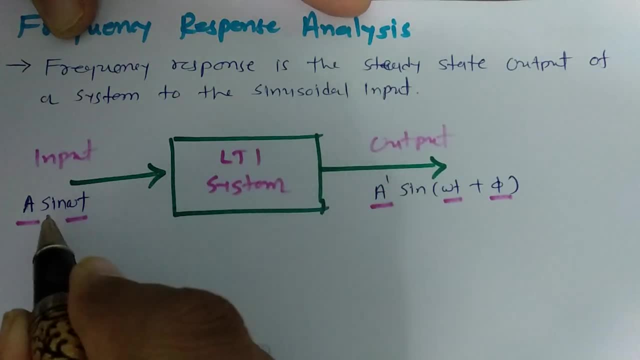 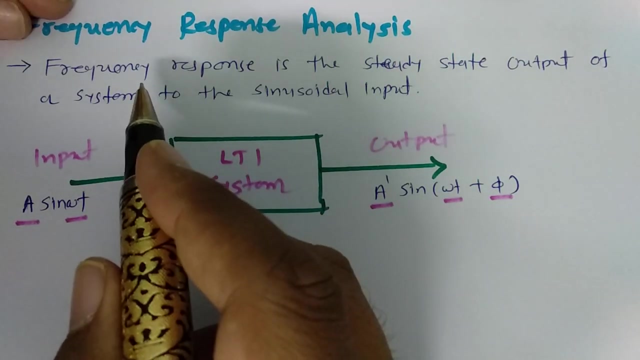 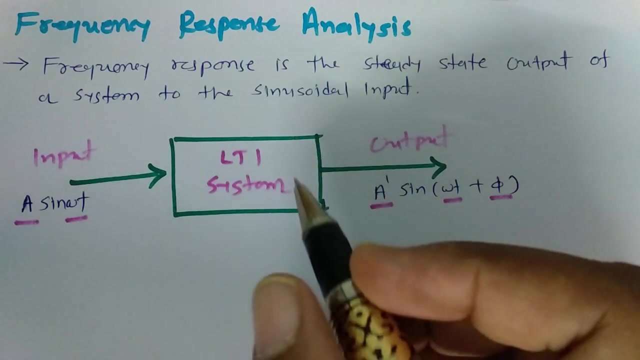 So here you can take input cosine as well as sine. Both are sinusoidal input only. So either you take cosine signal or you can take sine signal to give input. So what is frequency response analysis? Frequency response analysis is steady state output analysis of a system, provided input is sinusoidal signal. So, as I have told, one LTI system is there where input 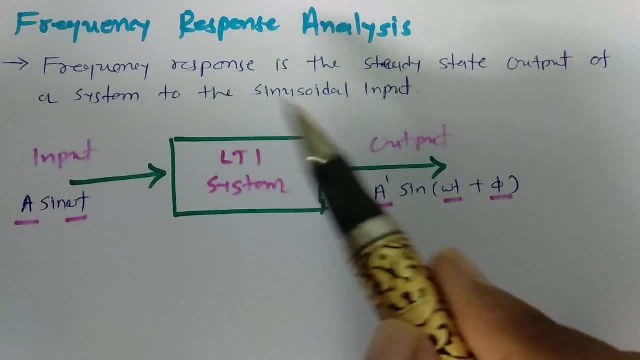 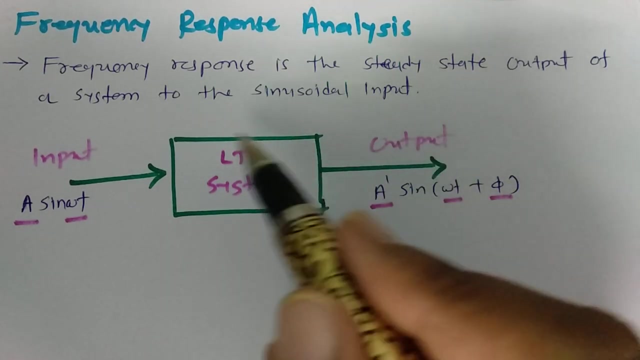 That is what sinusoidal input that one can see over here- A sine omega t, and output that is A dash sine omega t plus phi, where A dash is output amplitude that is getting changed because of this LTI system and phi that is a phase that is getting added because of this LTI system. 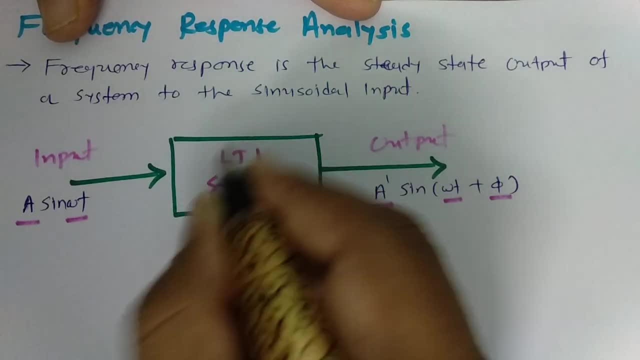 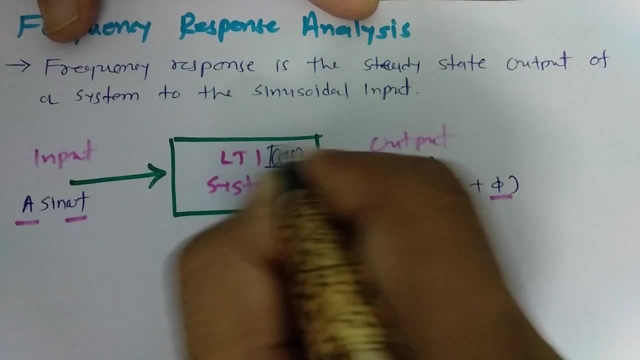 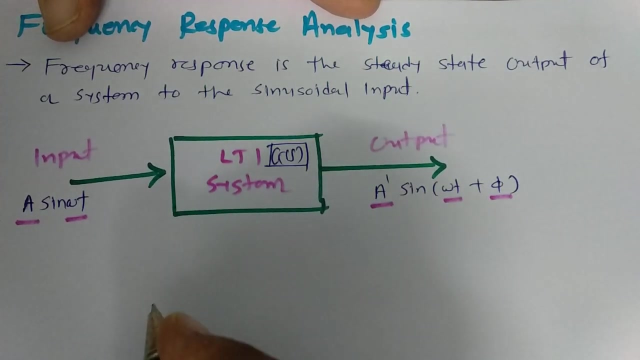 Now let us consider this LTI system that is having transfer function G of s in frequency domain. So transfer function of this system, that is G of s in frequency domain. So here, as I have told my input, usually we note it as RT, So input signal that is RT and that is A sine omega t. 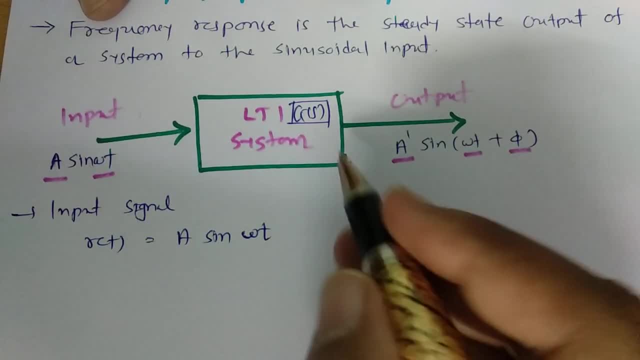 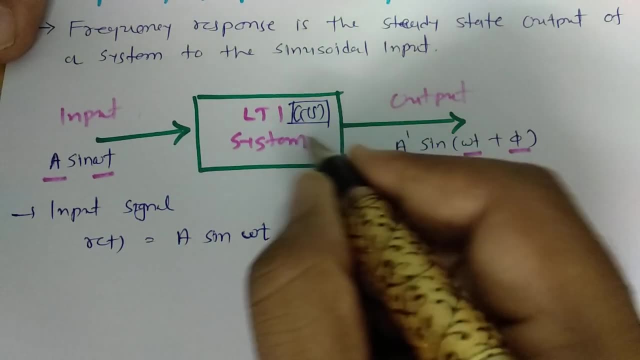 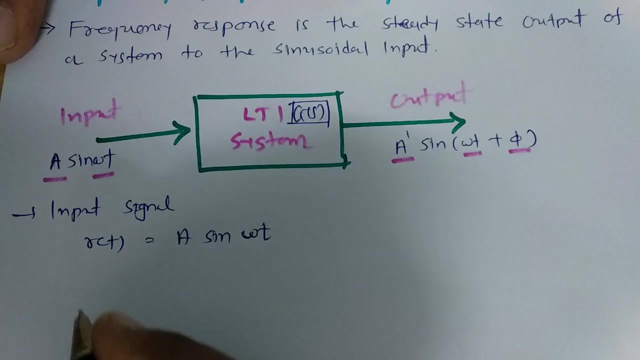 Now here I will be explaining you like see how this output amplitude, as well as phase, is getting changed. So we have systems transfer function. that is G of s. Now to have it in time domain, we need to consider: s is equals to G omega. 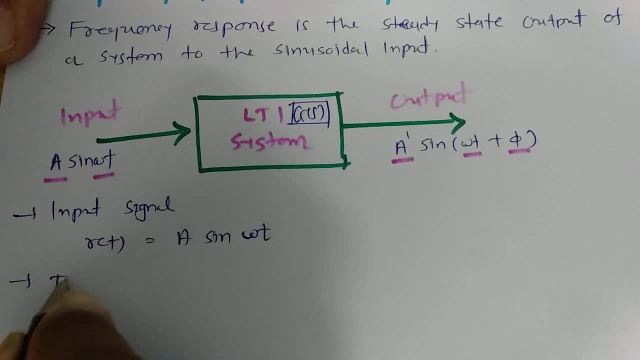 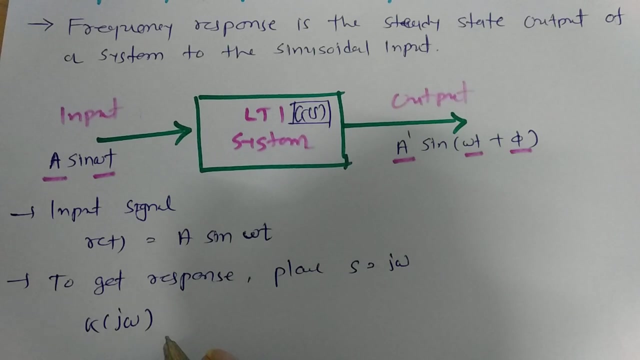 So here to get response, Place s is equals to G omega, So now we will be having G of j omega instead of G of s. Now, G of j omega, that is having two things: One is amplitude as well as one is phase. 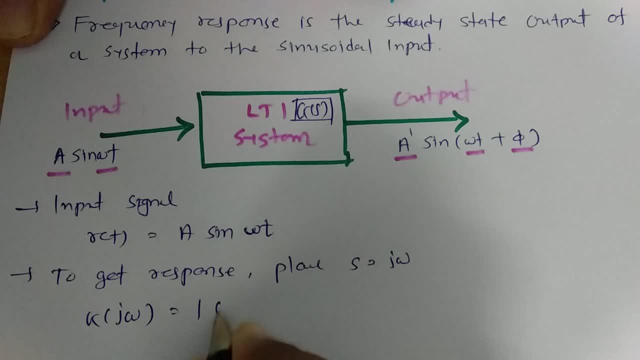 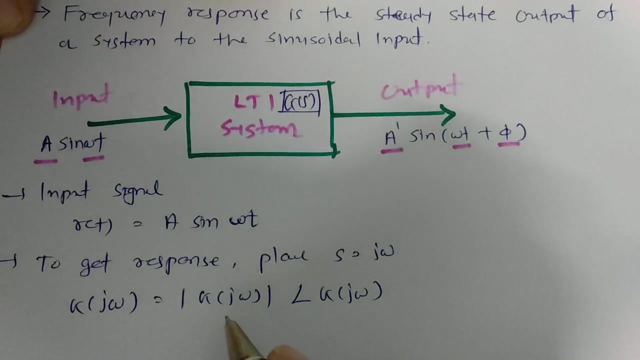 Now amplitude that we can represent as mode of G of j omega And And phase that we can represent as this phase of G of j omega. So, ultimately, we can represent this systems magnitude by this magnitude G of j omega and phase by G of j omega. 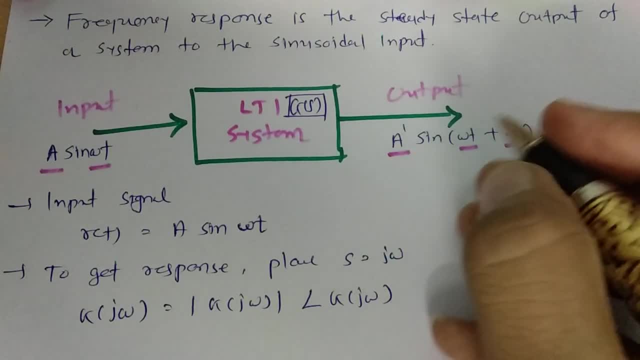 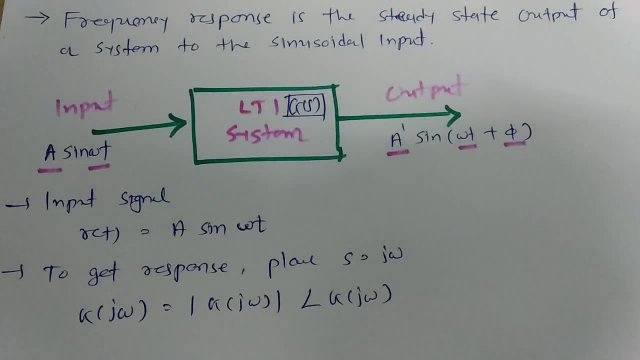 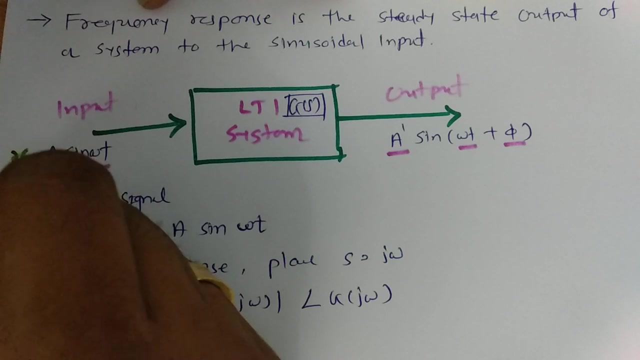 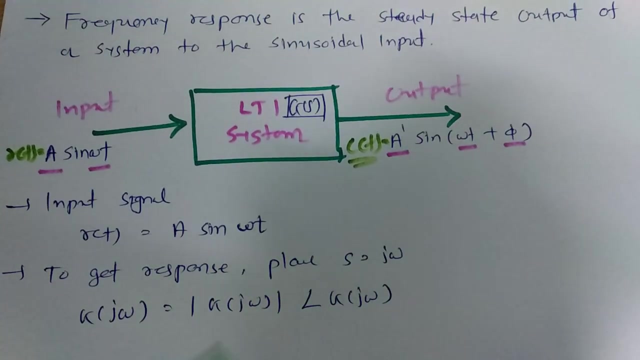 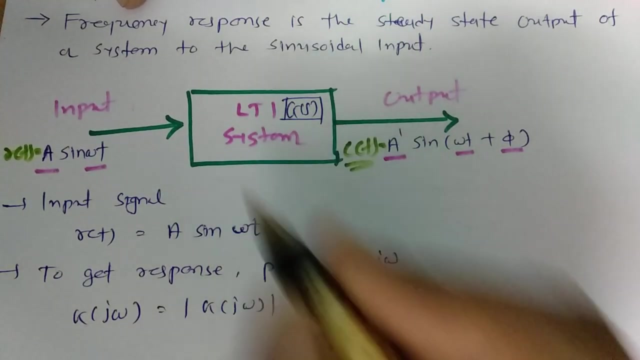 Now, as we know, output that we usually note down as C of t output- That is what we know- That we note down as C of t, see input that we note down as R of t, an output that we note down as C of t. so how to calculate C of t? C of t will be input into transfer function of this system. 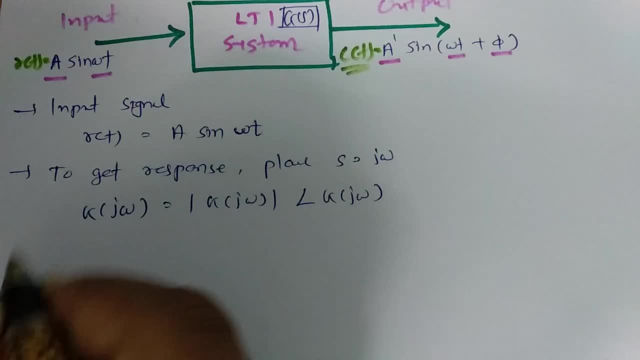 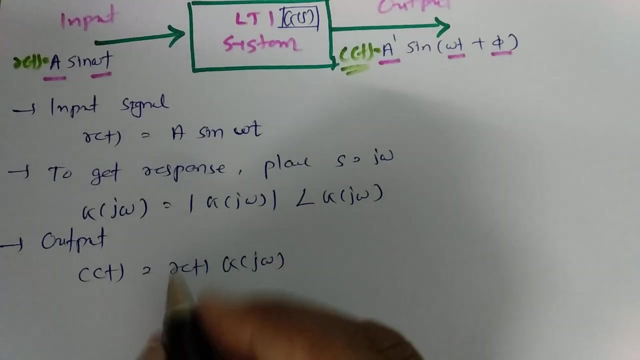 So now let us have output. so output that will be C of t and that is R t into G of j omega. now R t, that is a sign, omega t and this G of j omega, that is having two things: one is magnitude, so mode of G of j omega and angle of G of j omega. that is phase. 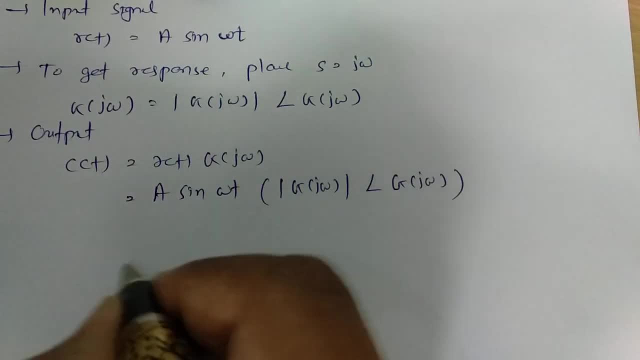 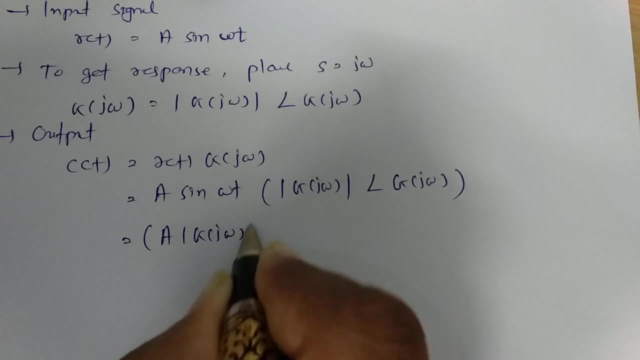 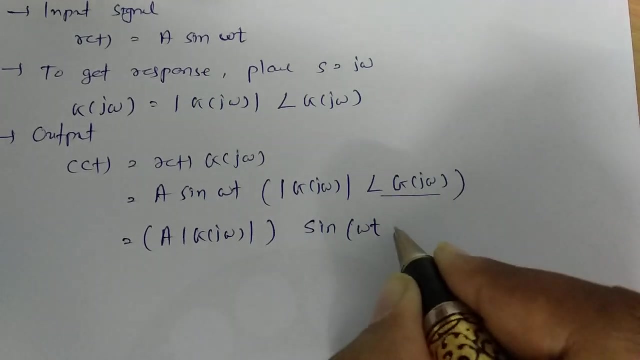 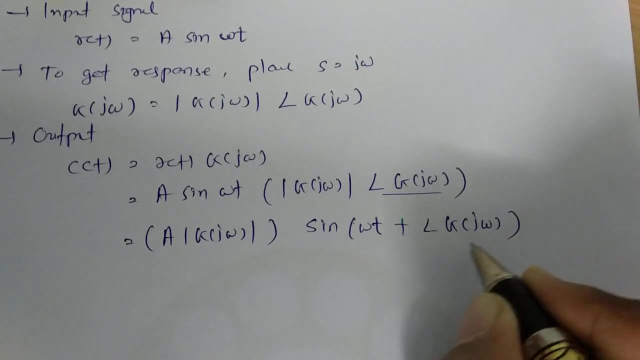 So if you further simplify, So if you further simplify this, then this will be having magnitude that is a into mode of G of j omega into now sign of omega t and because of this phase is getting changed. so I am just writing it angle: G of j omega. so that is what phase added because of system. 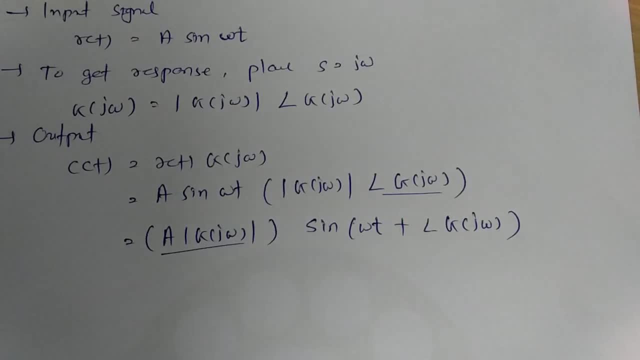 So resultant of this that I am considering as a dash resultant of this, So that is what a dash. So that is what a dash, So that is what a dash into. sign of frequency is omega t, and this is what I am. 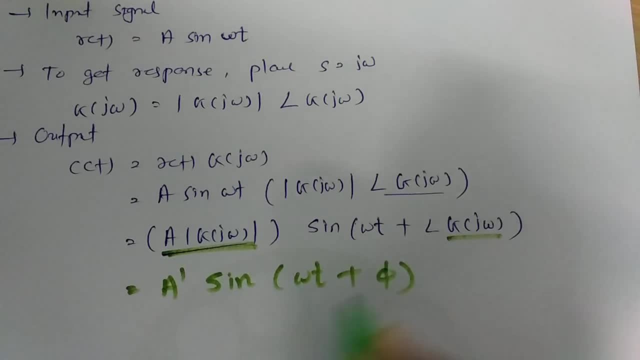 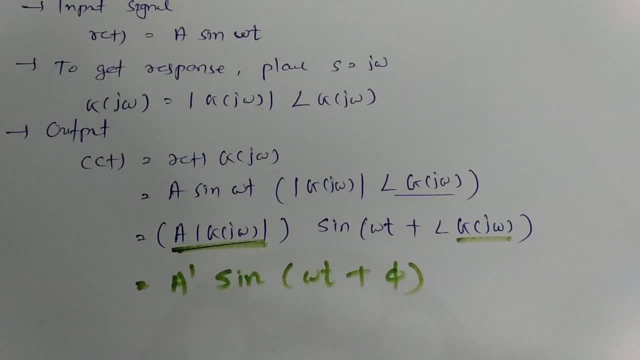 considering as phi, so omega t plus phi. so when we see frequency, response analysis is what we observe, as we have the change in amplitude and change in phase. so here our analysis is that will be based on this change in amplitude And this chance in amplitude. So our analysis is that will be based on this change crossover and the change in amplitude in phase, so that we can definitely consider fix that because the особенно to be done in problems of 130 testba- yes, ok, now the formula of very Elmer's- are seen that all have two problems which are value pi. 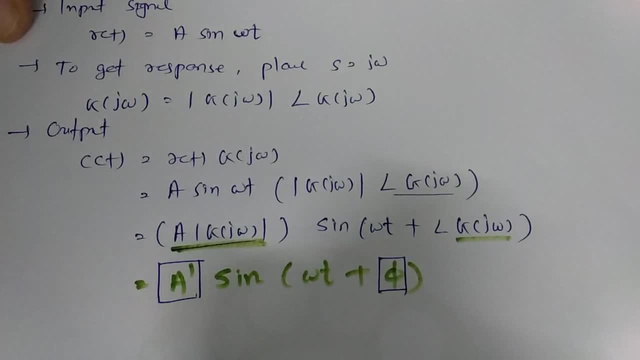 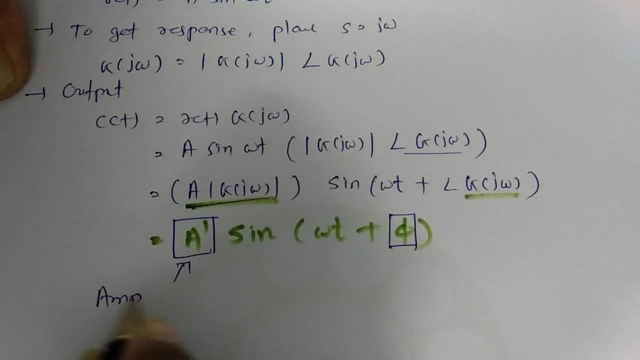 Plus 0. Displ güle주 rainbow matching the cold temperature. plus 0 is 10 to 14.. covering cold temperature can control temperature or excess temperature of 5000 watts. change in phase, So amplitude is getting changed because of system Amplitude changes due to. 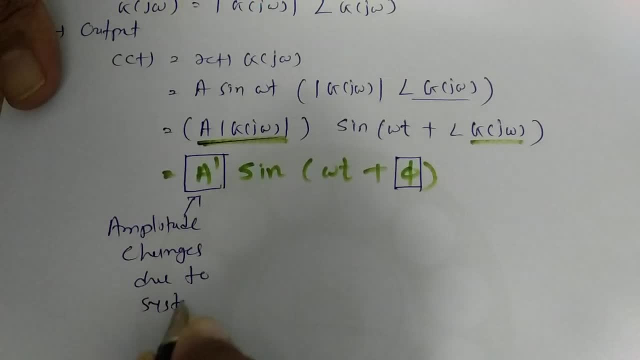 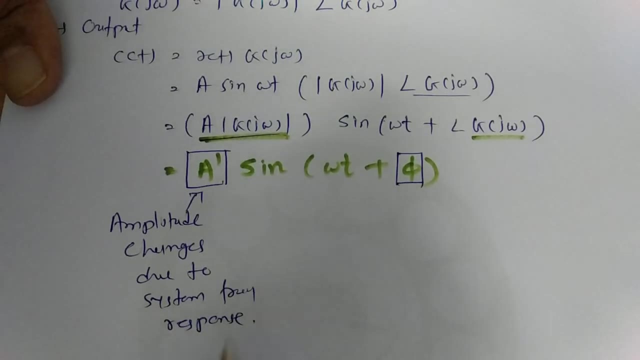 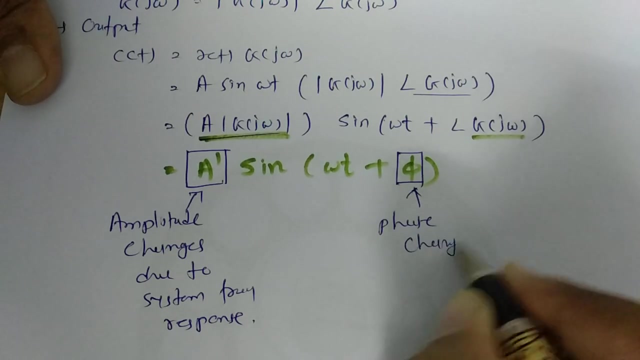 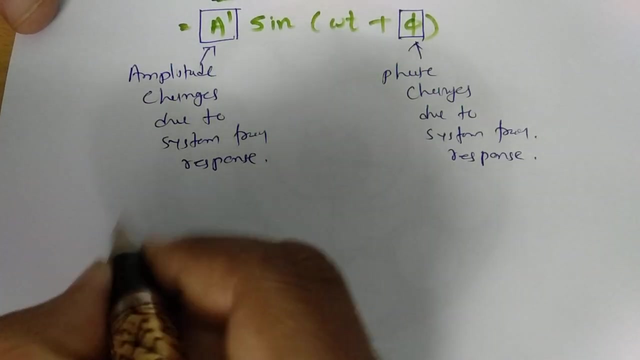 system response, System frequency response, And here this phase changes due to system frequency response. So this is what we are dealing with, to analyze, And when we study this analysis- frequency response analysis- there are various techniques in control engineering, So I am just listing out those techniques to analyze. 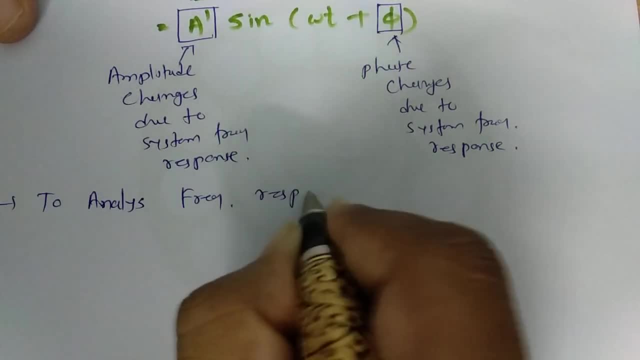 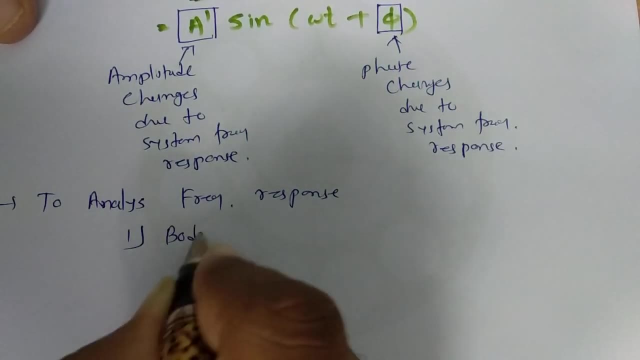 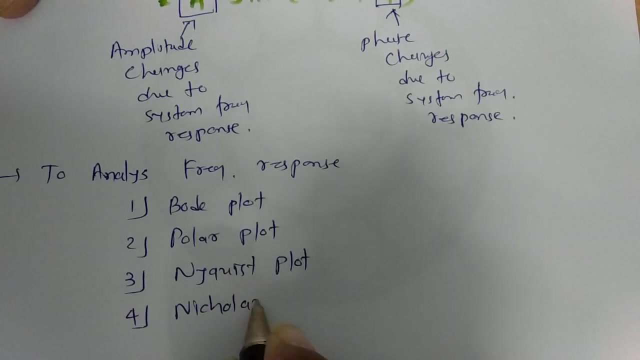 Frequency response. We have different techniques. First is body block. We have different techniques. Second is body block. Second is polar plot. Third is Nyquist plot And one more method that is there, that is by Nicholas Chart. So in my playlist I have explained these methods: body plot, polar plot and Nyquist. 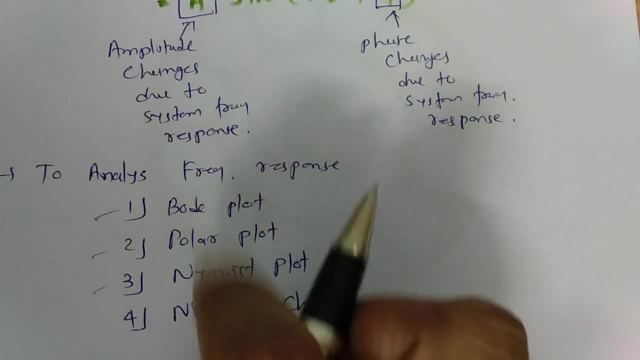 plot. Now, before I go for explanation of all those methods- body plot, polar plot, Nyquist plot- First I'll be explaining frequency response analysis by different parameter calculations like bandwidth, maximum peak, overshoot, resonance frequency for second order system. 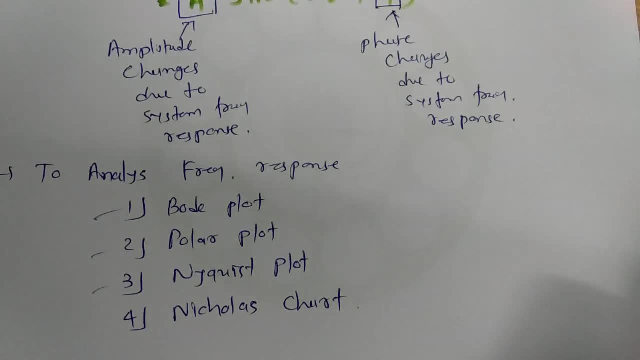 So I'll be explaining second order systems response by calculation of all those parameters in next few sessions. So stay tuned with this channel to understand frequency response calculation, And after that I'll be going to explain these methodologies, like body plot, polar plot, Nyquist plot. So that is what you'll be finding here in sequence.